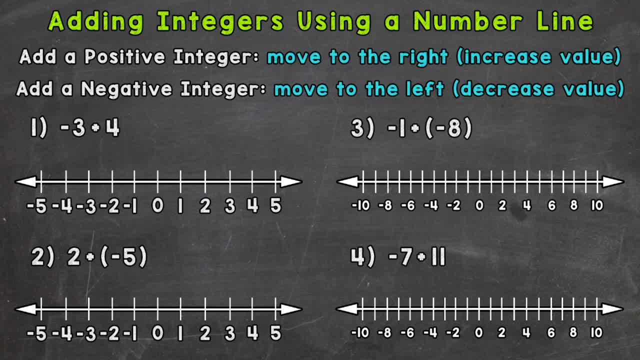 Let's jump into number one, where we have negative three plus four. So we're starting at negative three and we are adding a positive four, So we are increasing in value. We are going to move to the right. So let's start at negative three here. 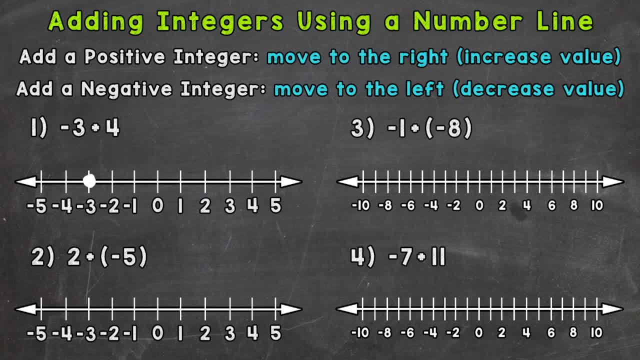 And we are adding a positive four. So four spots to the right, So one, two, three and four. So we end up on a positive one And that's our answer. So the answer to negative three plus four is a positive one. 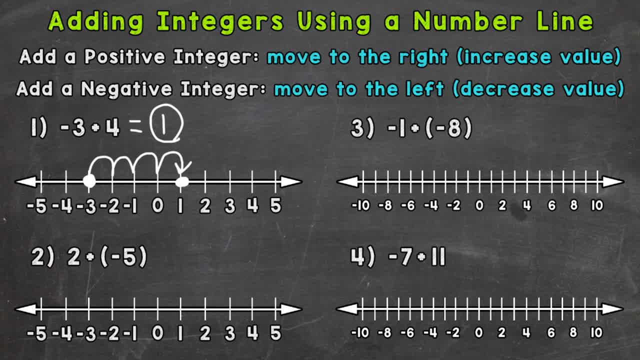 On to number two, where we have two plus negative five. So we're starting at a positive two and we're adding a negative five, So we are decreasing in value. We need to go to the left for number two, So we'll start at positive two. 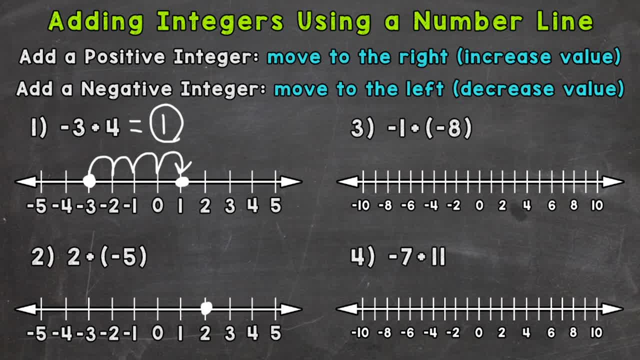 And we need to go to the left. five to represent adding negative five. So one, two, three, four and five. So we end up At negative three And that is our answer. So two plus a negative five equals negative three. 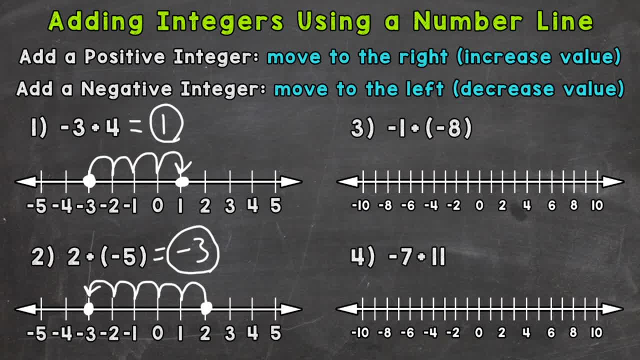 On to number three here, where we have negative one plus negative eight, So two negative numbers there And we are adding a negative integer. So we are going to decrease in value, which means moving to the left on the number line. So we'll start at negative one. 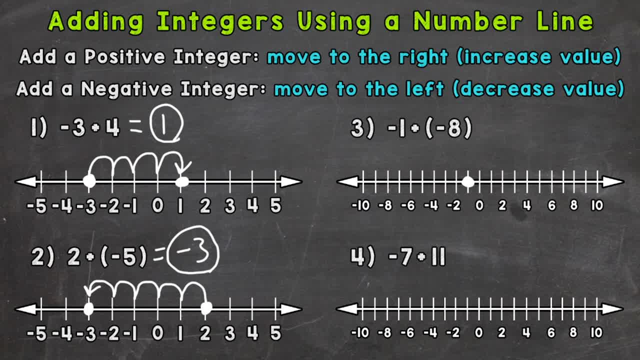 I only have the even numbers filled in for the number line because it was too jammed with all of the numbers there. So we are at negative one between zero and negative two there. So we need to move to the left eight spots to represent that negative eight. 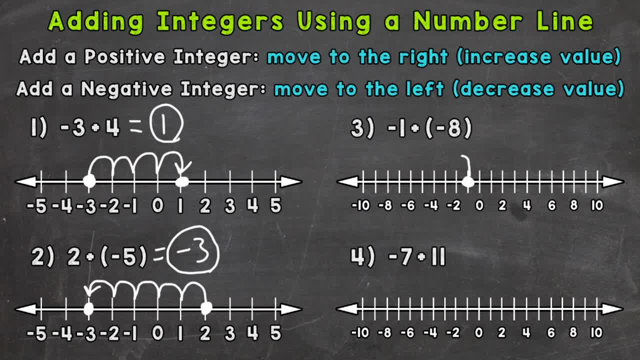 So let's start here: One, two, three, four, five, six, seven. One, two, three, four, five, six, seven and eight. So we end up at negative nine, So negative one plus negative eight equals negative nine.